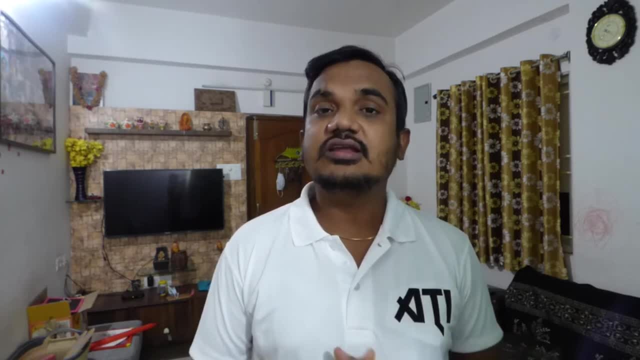 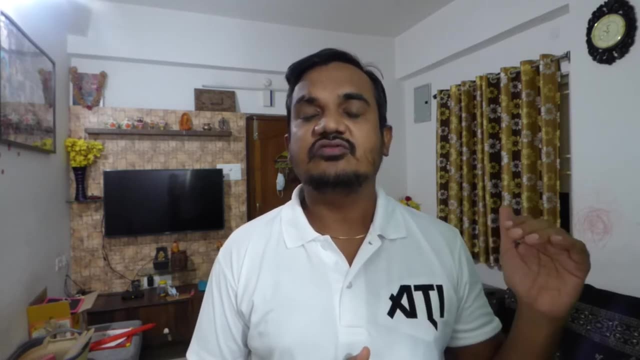 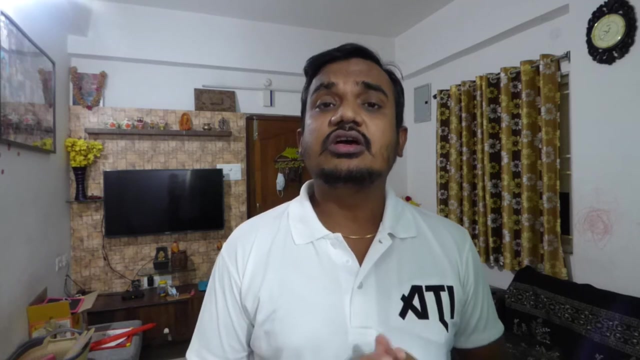 called linear sequential model. So if you have seen the last video, like we have certain phases in development, software development lifecycle, like we have requirement system investigation, we have requirement analysis, design, coding, testing and release and maintenance. So in waterfall model we used to follow the waterfall model. So in waterfall model we 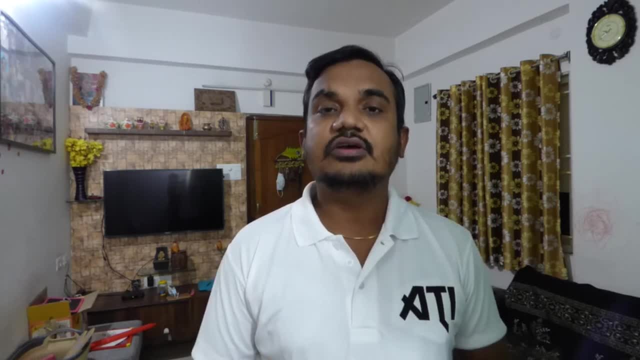 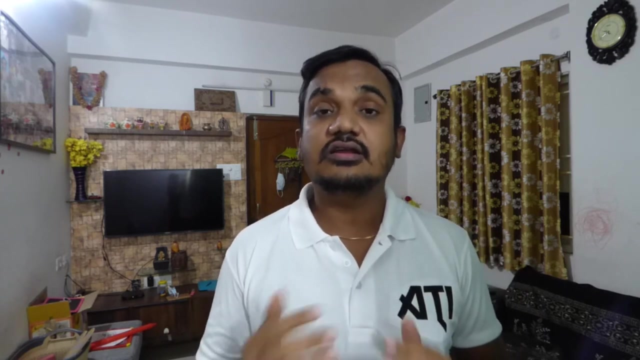 used to follow all these process. all these phases step by step, in a linear, sequential manner. So this is the reason it is called linear sequential model as well. So it's like waterfall, like from top to bottom. all the phases are in linear, sequential manner. So that's the reason it's like ladder, Okay. 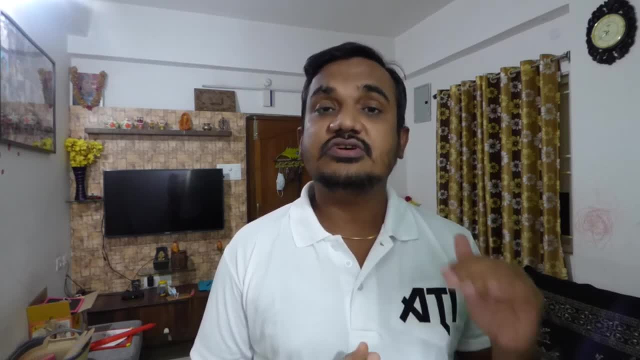 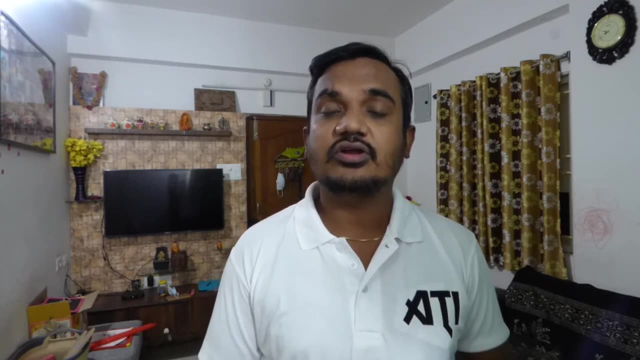 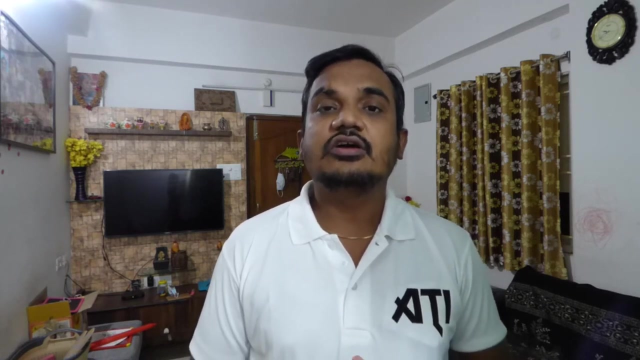 so once until unless, if one first phase is not completed, we cannot jump to the next phase. So that is the important concept behind this waterfall model, And we cannot come come back from the next step to the previous step as well. So we'll talk more about waterfall model in my PPT as well. So this is about the 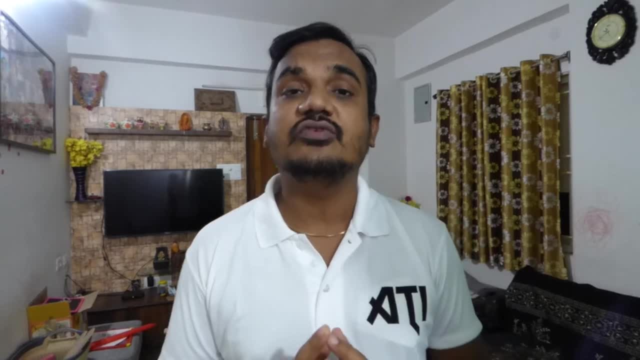 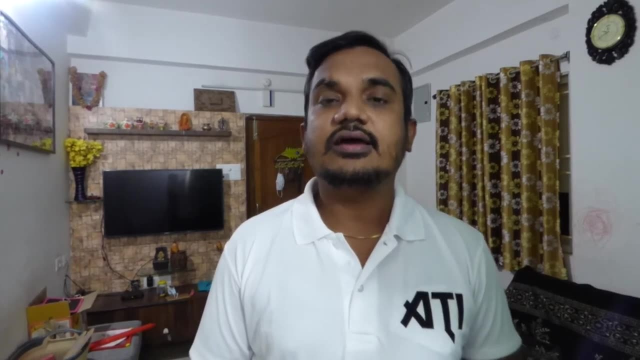 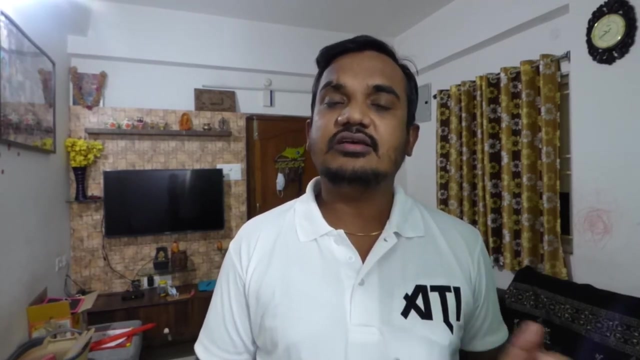 waterfall model and when to use. So when the project is very short, it's, it's not complex, then we can go for waterfall model. And another thing is, if requirement is clear, then we should go for waterfall model. So I'll take you to my system and I'll show you in PPT like what are its. 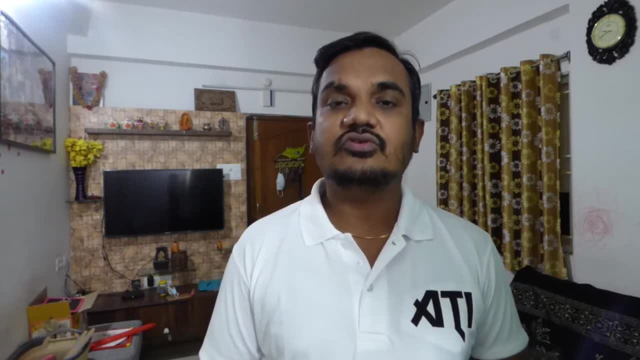 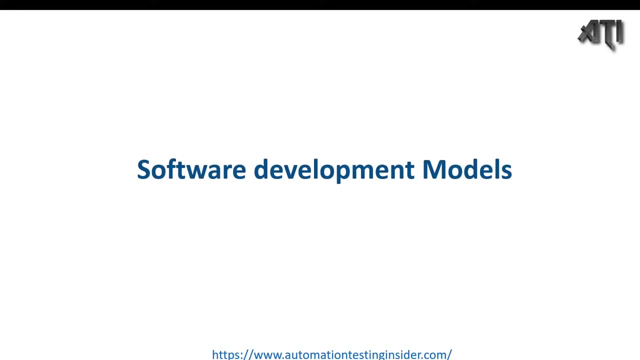 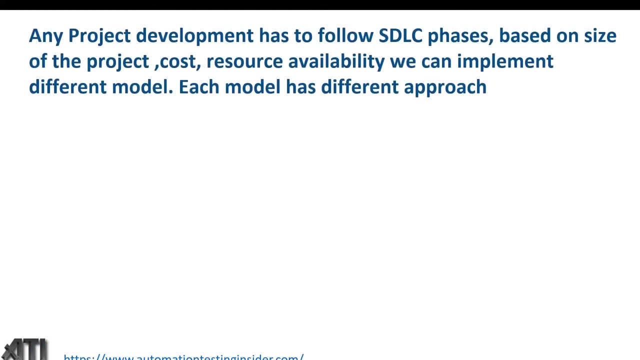 advantages and disadvantages of waterfall model. So let's get started. Let's talk about what are the different software models we have in the industry. make any design development as to follow as VANC phases. so we talked aboutahaha phases: requirement analysis, design, code design, data capture and other uncertainty Design- This all process. 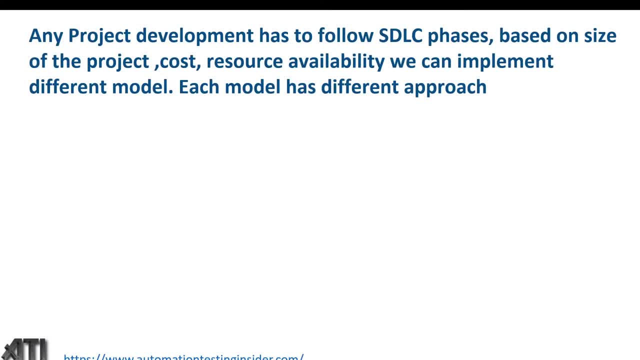 analysis, design, coding, testing and release and maintenance, and based on the size of the project, cost, availability. we can implement different models as per sdlc phases, and each model has its different approach, guys. so let me talk about what are the different models. we have waterfall model, which is called linear sequential model. we'll discuss about. 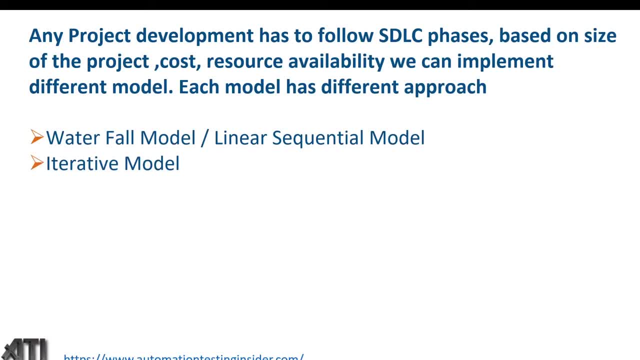 today and iterative model, spiral model, v model, agile development model and agile development model is very frequently using nowadays and it's very important protect a prototype model, hybrid model and derived model. so these are the different models we have in the industry to develop any software and mainly today we'll focus on waterfall model and in coming days. 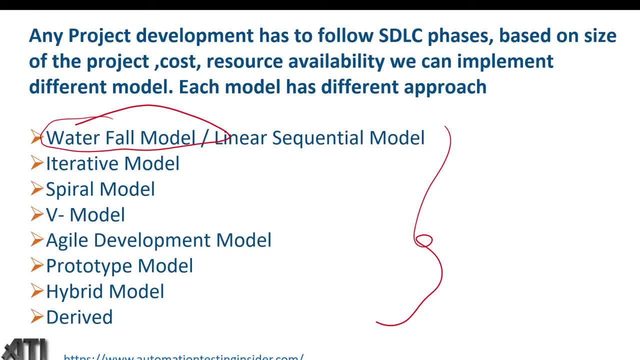 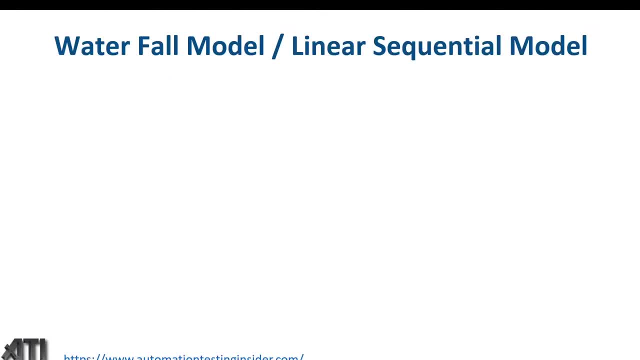 i'll explain each and every models, whatever we have listed down here. so let's get started with the waterfall model. so, as i have discussed earlier, the waterfall model illustrates the software development process in a linear, sequential flow. in the next slide, i'll show you, like, what do you mean by this? 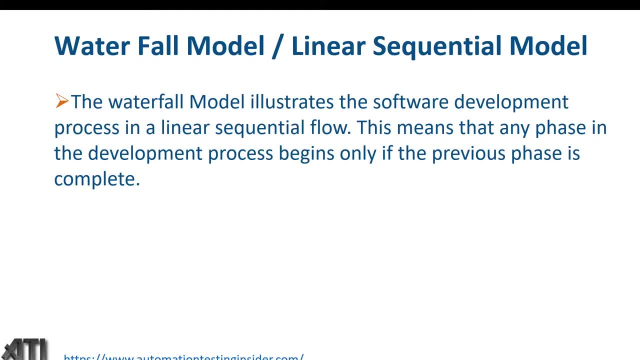 linear sequential flow because there are different phases in waterfall model, like sdlc, and that is in linear sequential flow, linear sequential manner. this means that any phase in the development process begins only with the previous phases complete and waterfall model is sequential model that divides software development into 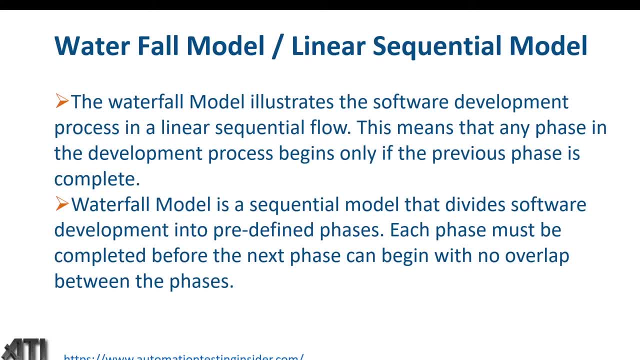 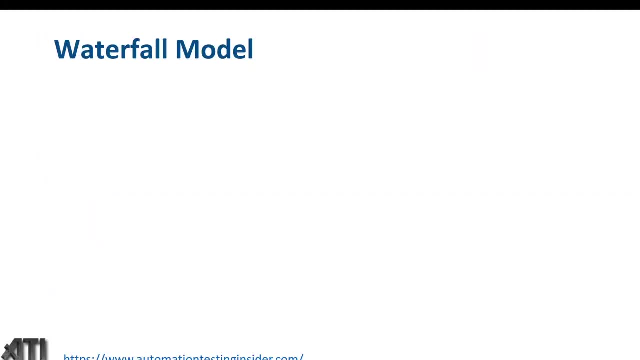 predefined phases. each phase must be completed before the next phase can begin, with no overlap between the phases. now let's understand with the help of uh representation guys. so i'll create a draw diagram so that you can understand it better. so, as we have discussed, different phases are there in the 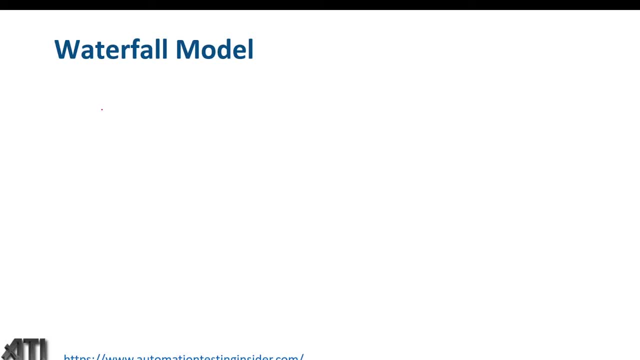 software development life cycle. like we have requirement analysis, design, so these are the different phases in waterfall model. like we have requirement analysis and you can say feasibility study as well, and we have design, design, coding, testing, release and maintenance. so the flow is like once requirement analysis and feasibly feasibility study is done, so the 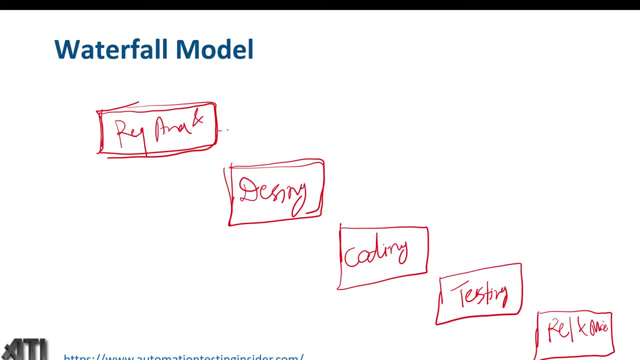 requirements will be reached. the flow will be like this. then only we can jump to the next part, design part. and once design is done, design will be done by the, the architect, who designs the complete framework architecture. and once design is done, based on the requirements, then developers will start coding, implementation, or coding will be started at that. 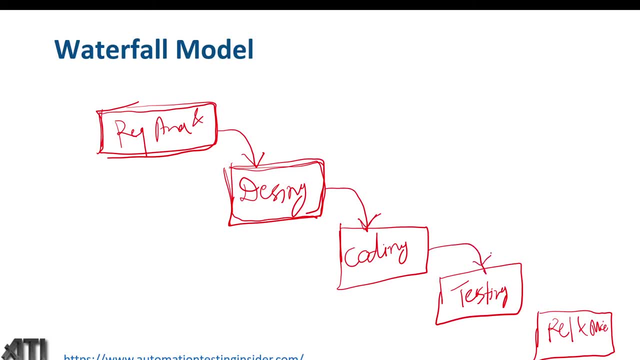 time and then once coding is done, then tester will perform the testing and at this point, will perform all kind of testing, all kind of system testing, uh, all levels of testing, and then, if anything, uh we, if we get any defects, then we'll revert it back to our coding team developers and they 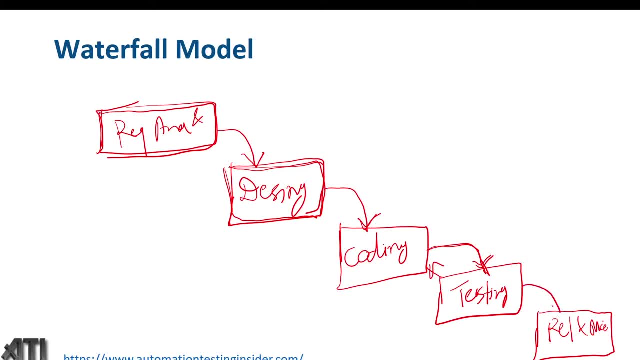 will fix the defects and then, last is release and maintenance. once testing is done, everything is done, if everything is working correctly, then we'll deploy the product. so this is how it looks like the waterfall model, phase by phase, and it is linear, sequential flow because, uh, from requirement analysis we are going to design, then coding, testing and maintenance. so this 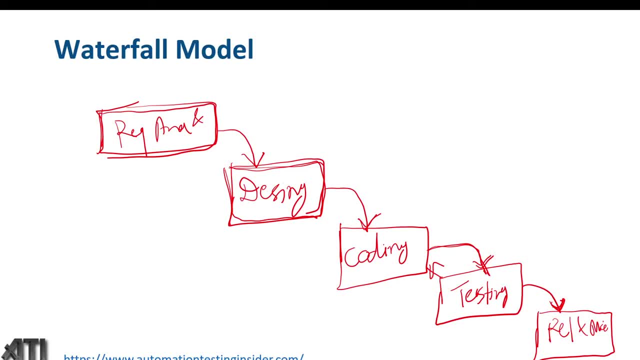 is: uh, in a, in in a flow, right in linear, sequential flow. so, if you see like waterfall, so waterfall looks like this: water is flowing. uh, it's flowing from the top to bottom like this, in a linear, sequential manner. so that's why, uh, waterfall diagram looks like this, only in this way. 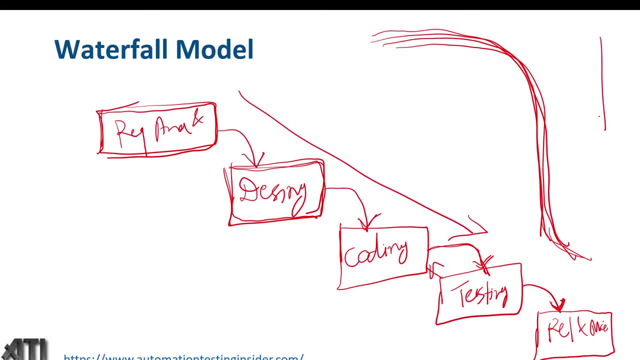 you don't see like this anywhere in the waterfall model. okay, so it looks like this because of it represents the waterfall and we cannot come back. uh, once our uh, the phases are done, right, so suppose requirement is done, feasibility study is done and we jump to the next phase. then we cannot. 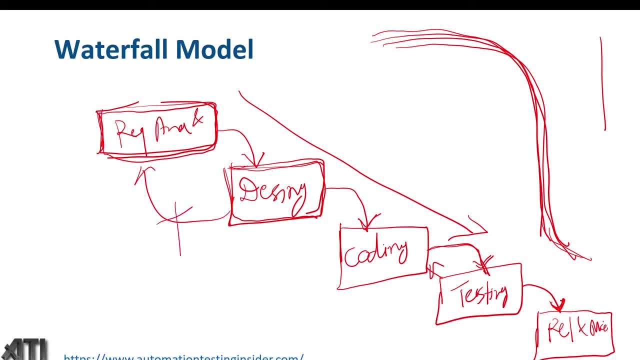 and change the requirements. so this is not possible in waterfall model. same thing over here. we cannot come back and design again from the implementation, the design part. similarly for testing as well. we cannot ask the developers to start the new uh testing for the new functionalities. so this is also not happening and the last as well. so this is useful for smaller projects. well in the 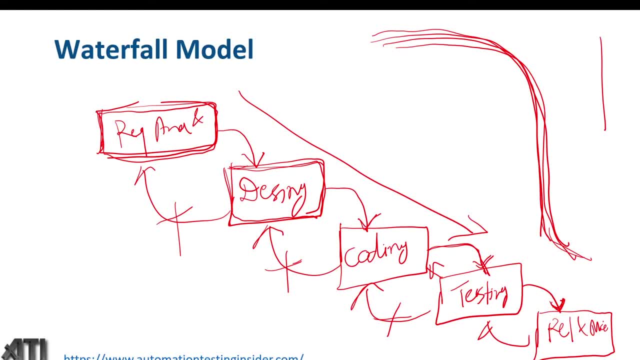 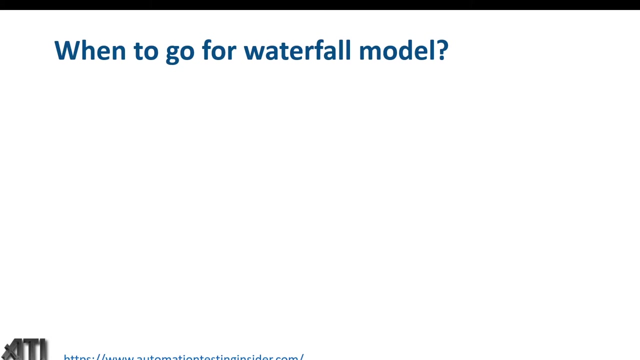 next slide, i will understand, we'll understand. like what? uh, when we should use waterfall model? yeah, and this is the oldest model, uh, traditional model, and this is also called basic model as well. so let's have a look. the next slide: so when to go for waterfall model? so when requirements are not changing frequently. 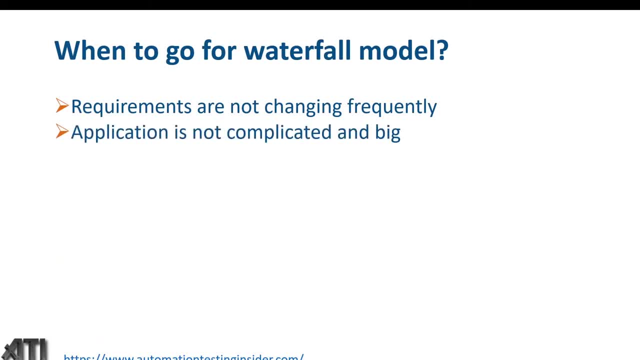 then we should use waterfall model. another thing is: application is not complicated and big, as i have discussed earlier. like it, it should be small project. then we can go for waterfall model. project is short and requirements is very much clear. environment is stable and technology and tools used are not. 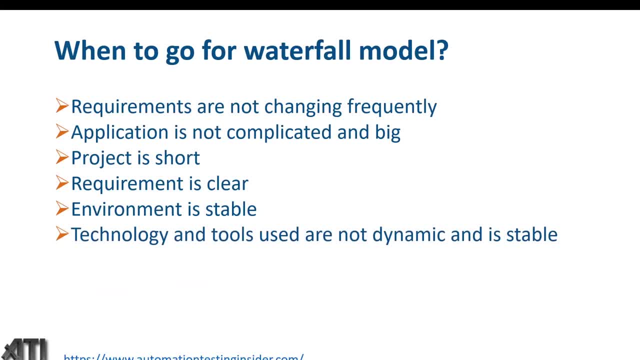 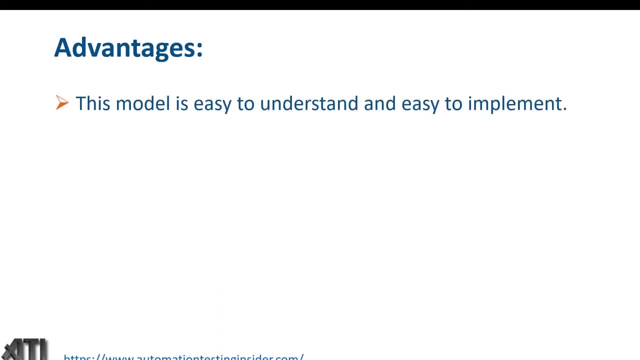 dynamic and stable. so these are the different uh things which for which we should go for waterfall model. then what are the different advantages of waterfall model? so this model is easy to understand and easy to implement. it is suitable for small and medium size projects. no change in the middle of the. 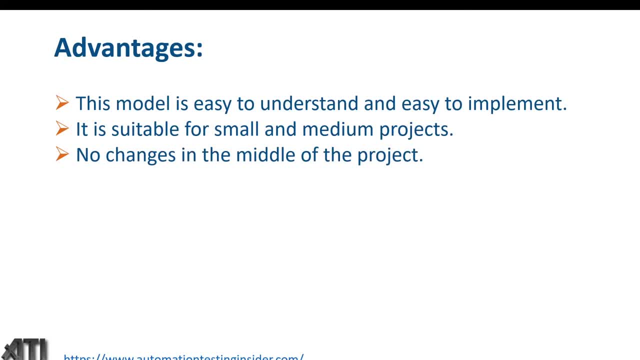 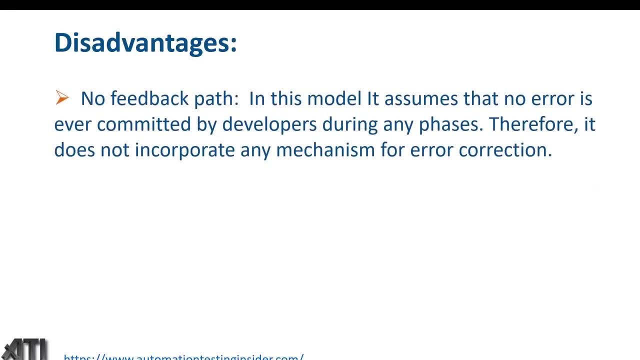 project. so there won't be any changes in the middle of the project. suppose we want to change any requirement, then it this model doesn't allow that. it is suitable for projects if requirements are finalized in the beginning. there are some disadvantages of waterfall model, like no feedback path. so what do you mean by this? 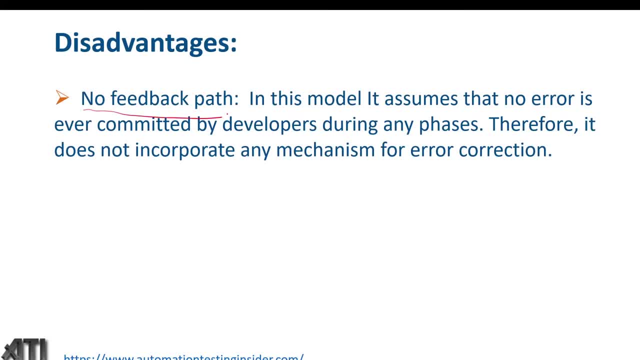 so in this model it assumes that no error is ever committed by the developers during any phases. therefore it does not incorporate any mechanism for error correction. so once everything is done, we cannot come back in the phase of waterfall model. once one phase is done, we cannot come back. 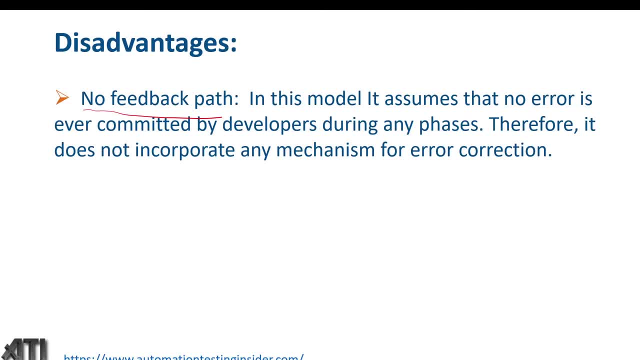 from the previous phase, next phase. we cannot go back in the phase of waterfall model. once a phase is done, we cannot come back from the previous phase. next phase it will be in the first phase of waterfall model, next phase to next phase, to previous phase. so there is no change. uh, chance of feedback.